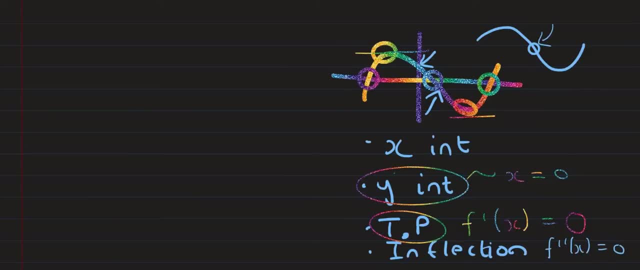 is equal to zero, And then x-intercepts. well, that's where you make y equal to zero. but this one's a little complicated because in grade 12 we have to work out three of the x-intercepts and it's a bit of a weird method and I'm briefly going to go over that method now with you guys. 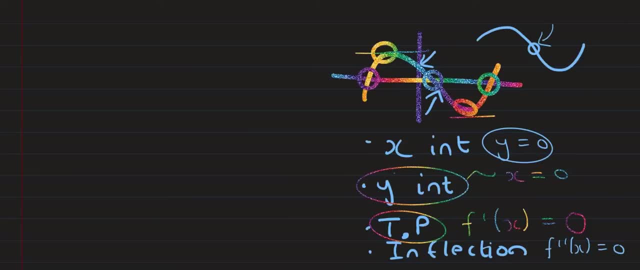 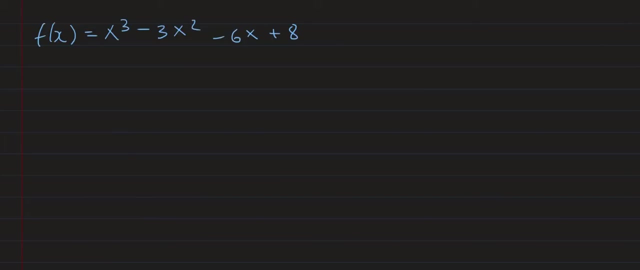 now. If you're still struggling with that, then please purchase the course on factor and remainder theorem. In that course I explain in detail how to work out the x-intercepts of a cubic graph In the process of drawing cubic graphs. this is the most challenging part, and in the next videos I'm 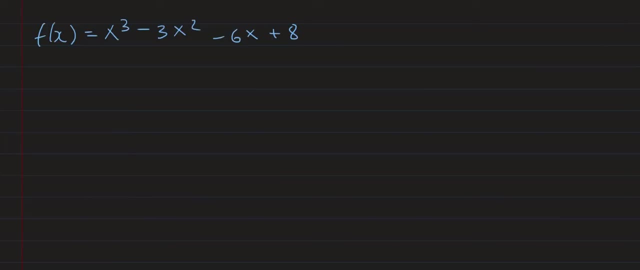 gonna do a couple of examples with you guys and go through the drawing process. But the most challenging part is the x-intercept. So remember to find x-intercepts. you make y equal to zero, so we start off like that. Now what you want to do is remember. we want to try to find three. 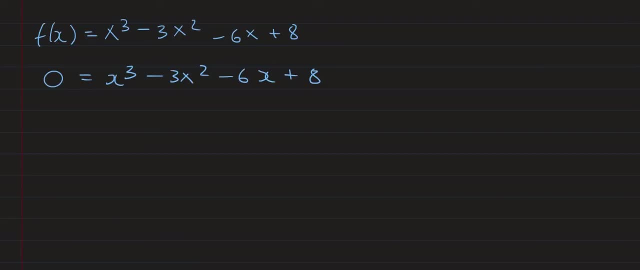 x-intercepts. Unfortunately, you have to guess the first one. so what you do is you keep choosing different values of x and t of t. Let's see our numbers. Two of these numbers are all the same, okay, So written right over here- which is zero. so let's do this. So let's just go with letter y, which is: 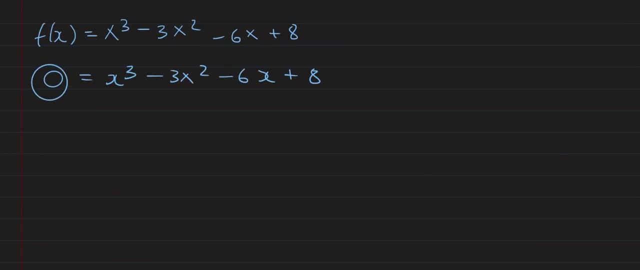 x that you plug into this equation until you get a 0 on the left hand side. So let's start by plugging in minus 1, for example. So it would say minus 1 minus 3 times minus 1.. So you see so. 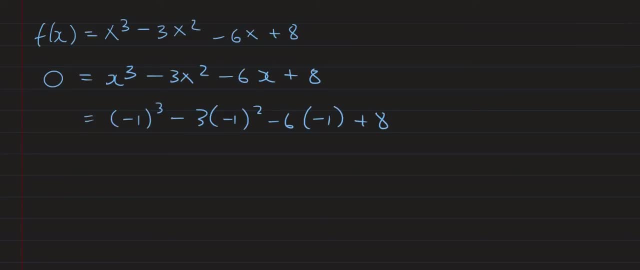 wherever there's an x, I'm plugging in minus 1, because I'm guessing that the first answer is minus 1.. You then go type all of that in on the calculator and that gave us 10.. So unfortunately, that one does not work. The fastest way would be to open a little template like this on your: 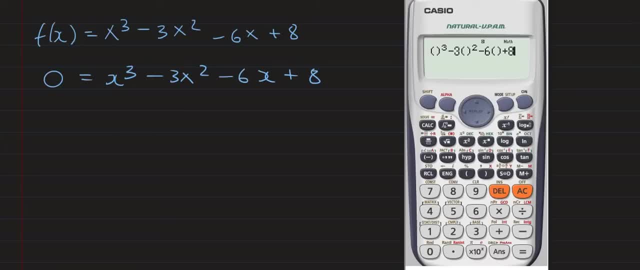 calculator where you can just go plug in different values for x. So, for example, I'm going to try the x value of 1 next. So what you do is you just backspace and you just keep going for, and you put in a 1 and you say equals. Ah there, we get an answer of 0.. So the first answer for our x. 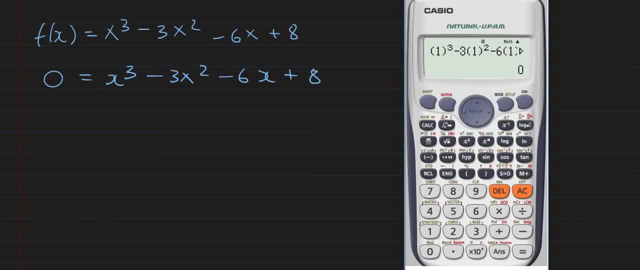 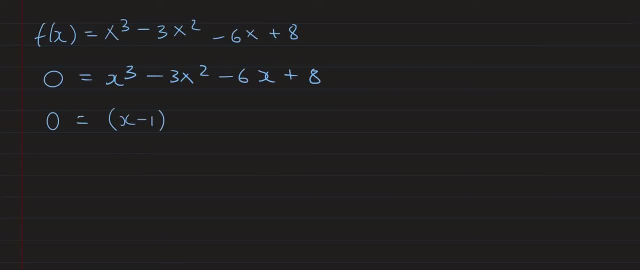 intercepts is 0. I mean is 1.. So if your x answer is 1, then in bracket form you have to remember that that means x minus 1. Remember because if I asked you to solve this equation you would say: oh well, x is equal to 2. 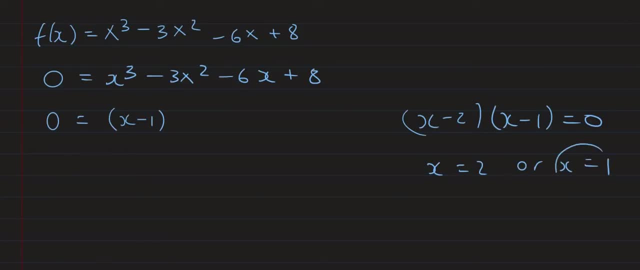 or x is equal to 1.. So notice that if x is equal to 1, then in bracket form it must be x minus 1.. Okay, now here's where this method gets a little bit weird. We know that if you had to divide or 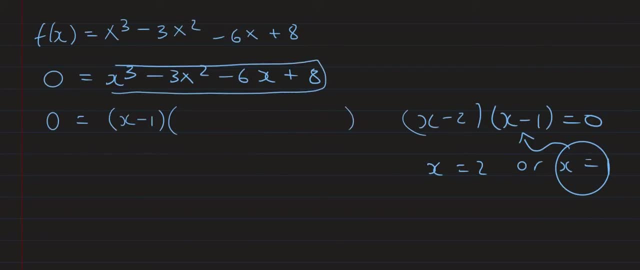 if you had to take x minus 1 out of this expression over here, you would have to take x minus 1 out of this expression over here. So if you had to take x minus 1 out of this expression over here, you would have to take. 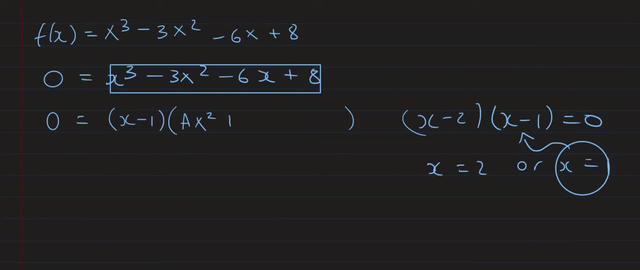 would be left with some type of trinomial. so we're just going to call it ax squared plus bx plus c, and the goal is to try find a, b and c. so a and c are very easy. if you had to try, if you had to. 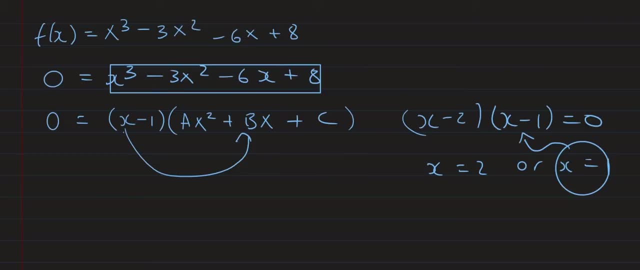 multiply these two brackets together. where would you get x to the power of three? we'll take some time at home and think about that, but the only place that that would happen is when you multiply these two terms together. so if you want those two terms to be the same as this one over here, 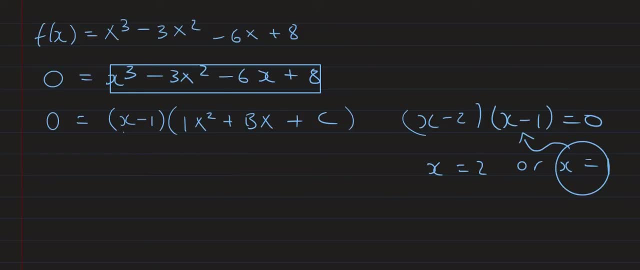 well, that means that a would have to have a value of one. now, the next thing is: where would we end up with a constant term like that if we were multiplying these two terms together? well, that would only happen over here, with that minus one and when you multiplied it with that. so we want. 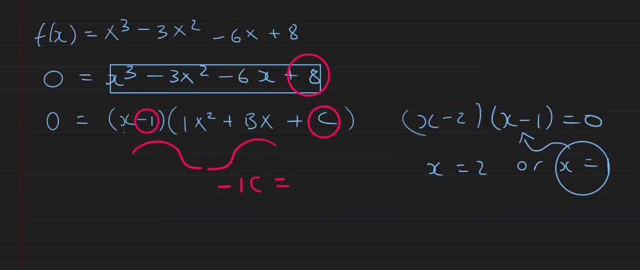 minus one times by c, and that should give us a value of eight. well, that means that c should be negative eight. now with the b value. here's where it's a little bit more complicated. so you are allowed to choose if you want to use the x squares or if you would like to choose the x's. it's completely. 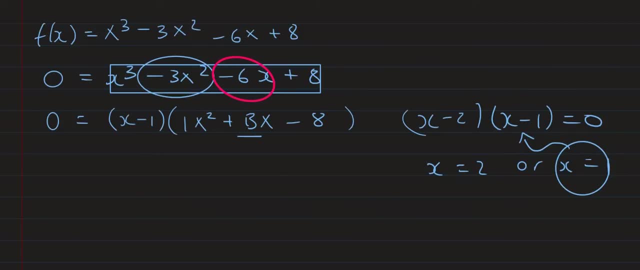 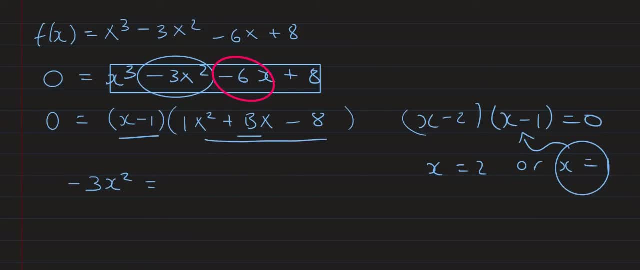